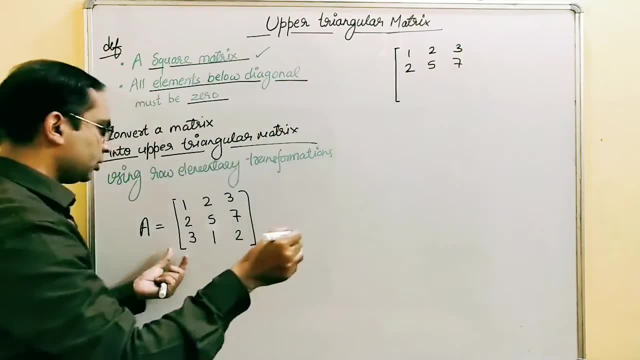 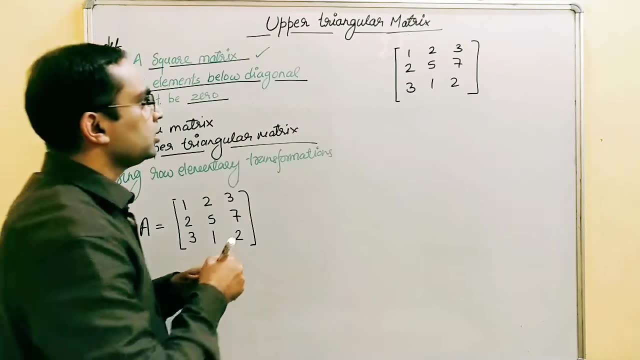 five, seven, two, five, seven, and then three, one and two, three, one and two, And we need to convert this matrix into a square matrix. So let's see how we can convert this matrix into a square matrix. So let's see how we can convert this into a square matrix. That means we want these three elements. 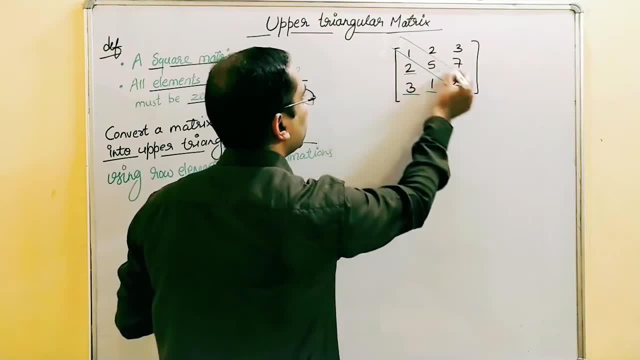 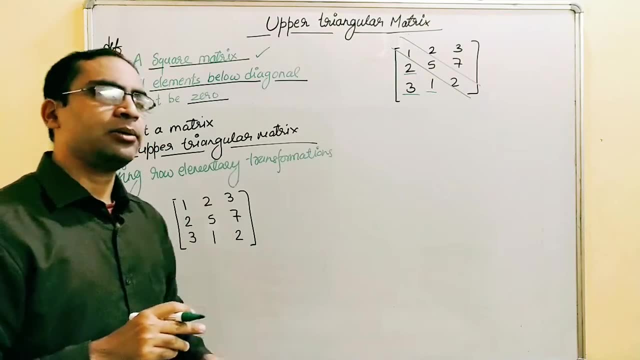 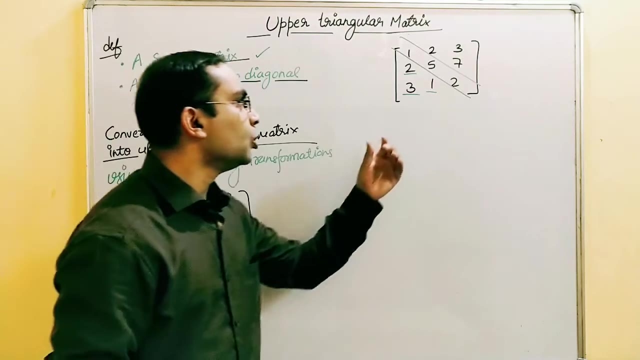 one, two and three, because these are below diagonal. We need to convert these three elements zero. So I'll tell you here three steps to convert any matrix into the upper triangular matrix. You need to remember these three steps. Step number one: we need to convert column by column. 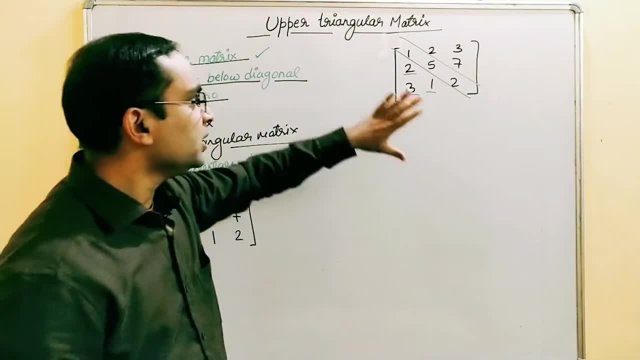 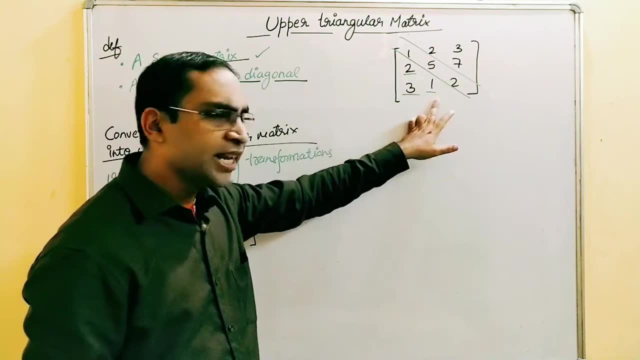 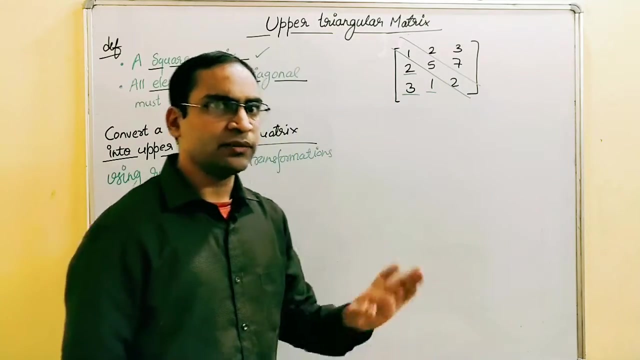 We need to convert elements column by column. So we'll start with first column and we'll convert all the elements of first column into zero. Then we'll move to the next column and convert all the elements of the next column into zero And similarly we will move further. Let's say if we have a four cross. 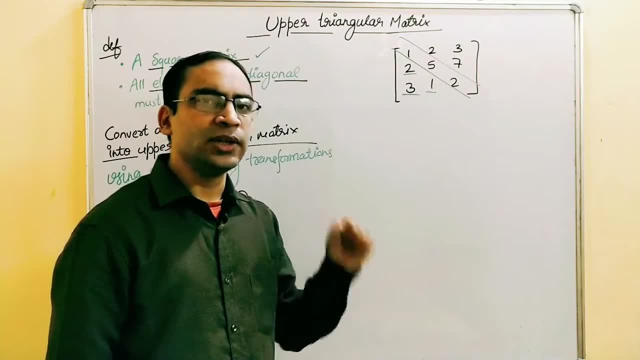 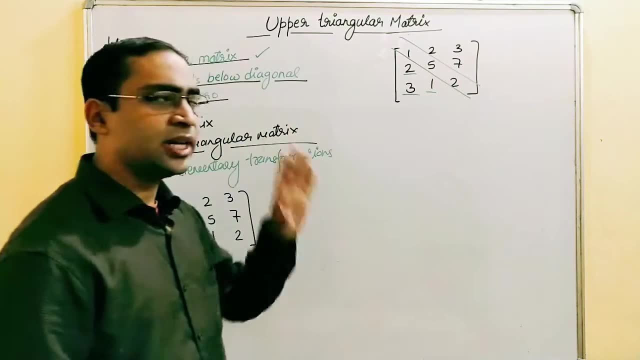 four matrix, then we'll convert all the elements of first column to zero, then second column to zero, then third column, and so on. So this is the way, the step number one, or we can say the tip number one: convert all the elements in the first column to zero. 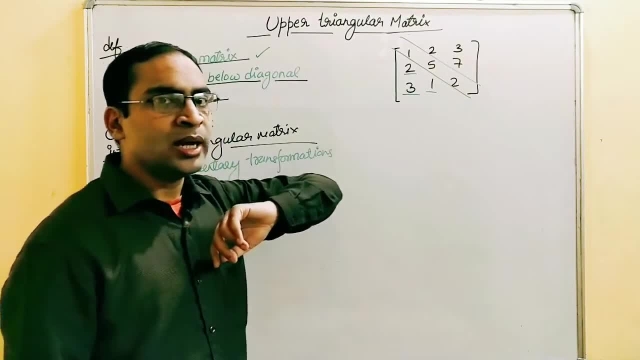 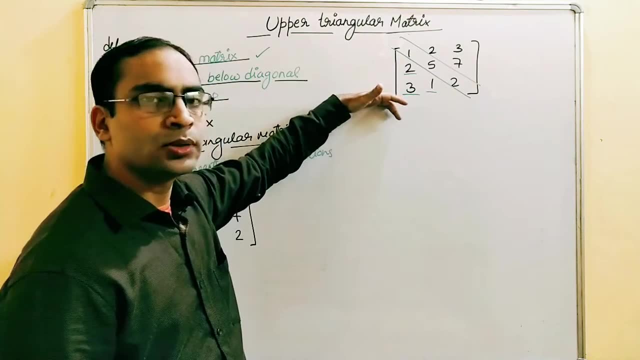 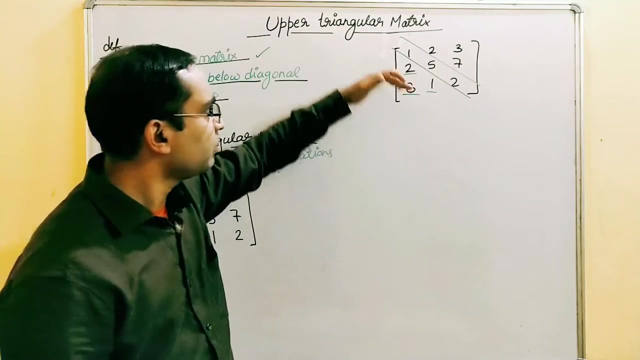 Then second and so on. Tip number two: while we convert all the elements in a column to zero, we should start from the top to bottom, So top row to bottom row. That means we will convert this element first and then this element, So we are moving from top to bottom. This is tip number two. or we can say: 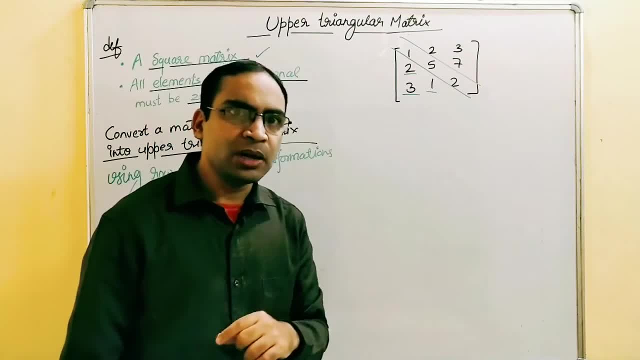 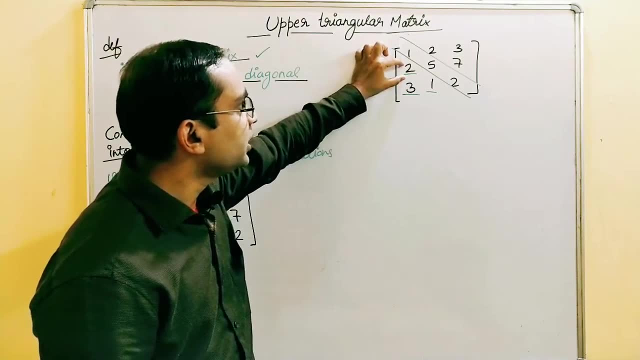 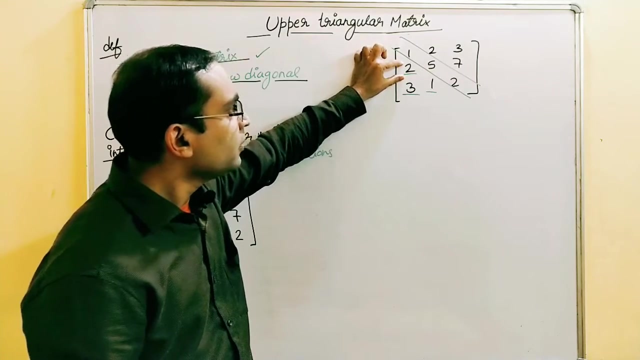 the step number two, Tip number three, or we can say: the step number three is we need to perform the next operation. Let's say: if you want to convert this element to zero, in which column it is? It is in first column, So we need to perform operation from first row, Right? So let's say: 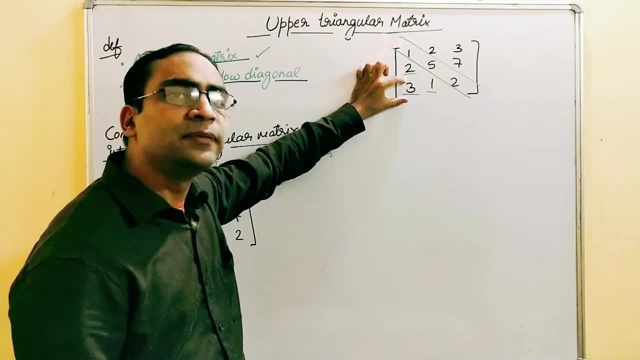 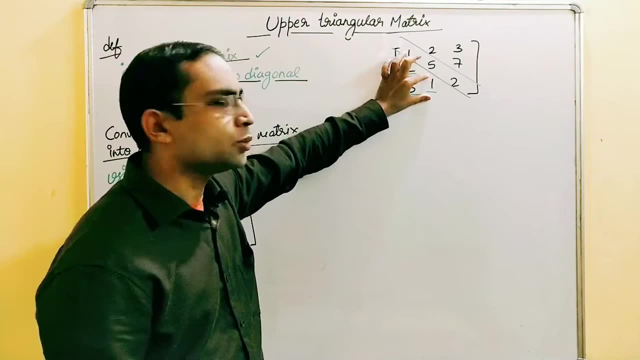 if we want to convert this into zero, This is in which column. This is in first column, So we need to perform operation from row number one. We need to convert this into zero, So this is in which column. This isn't column number two. 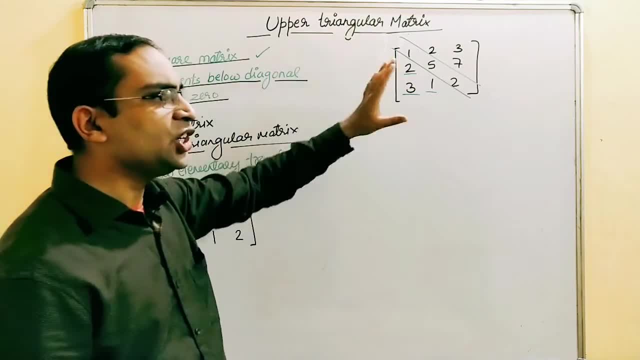 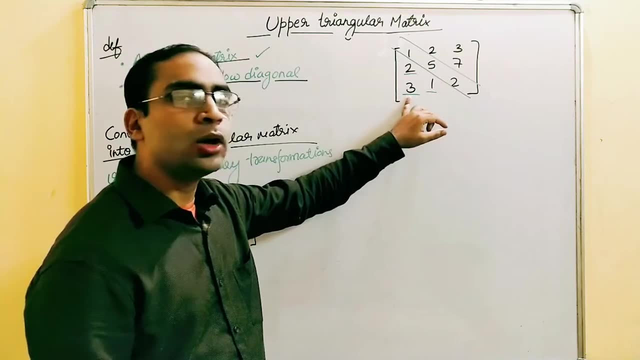 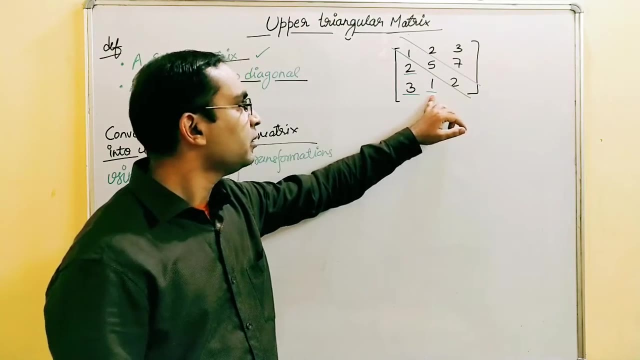 with row number two. right, so operations will be performed with the row with a number of row, such that the element is belonging to that particular column. so that means if element is in column number two, then to convert it to zero we will perform operation with row number two. so let's start. we'll have to take 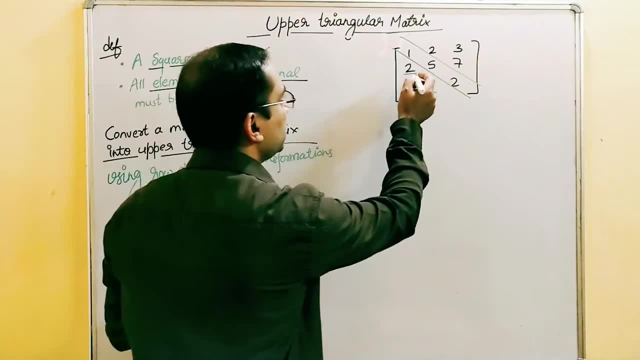 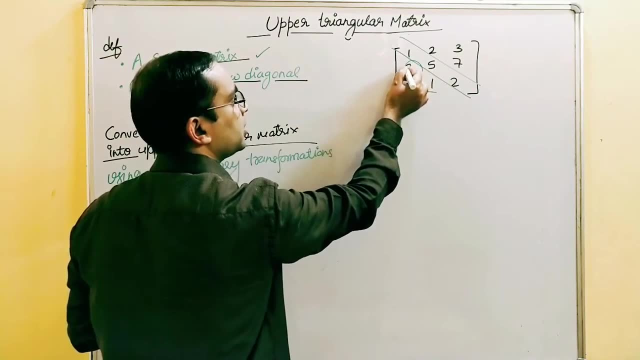 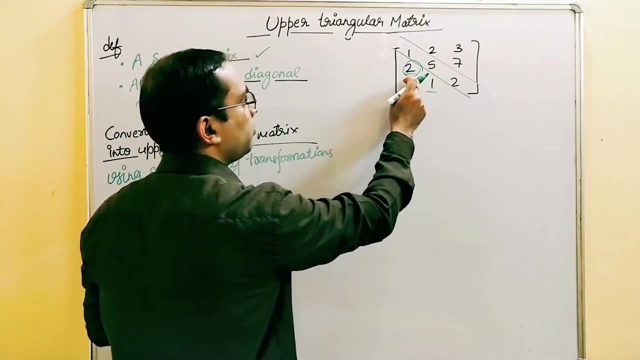 care of these three steps. so, according to this, we need to start from leftmost column and we need to start from top to bottom. so we will be converting this to two. zero first now and, yes, the tip number three. this is in column one, so we need to operate with row number one. so what operation we will be requiring? we 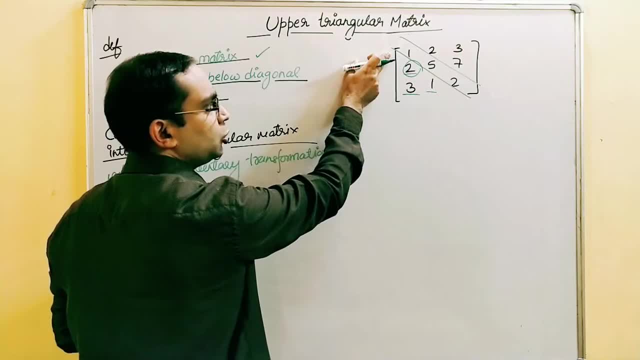 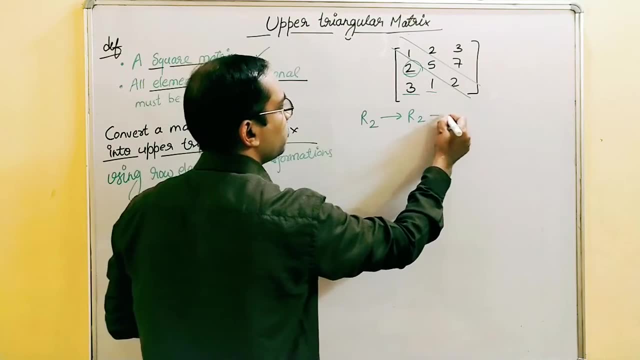 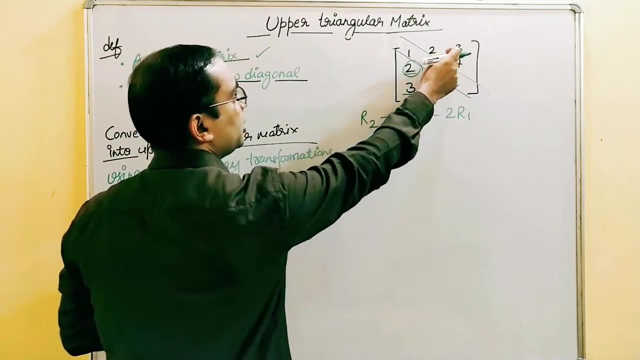 can multiply in row number one 1 by 2 and then we can subtract. so the operation will be: row 2 will be converted by row 2 minus twice of row 1. so this is the operation. operation we need to perform twice multiplication into row number one and then we'll subtract this. 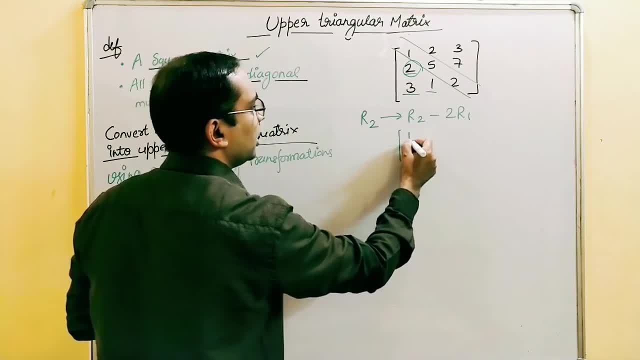 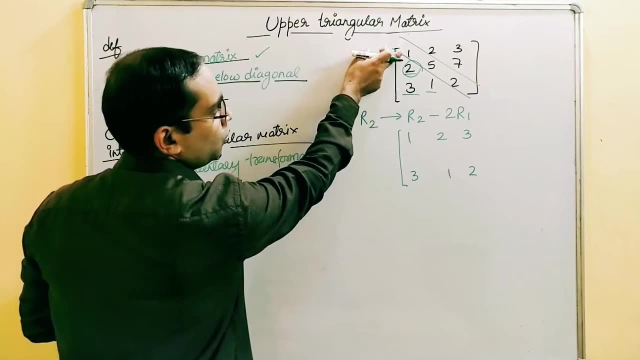 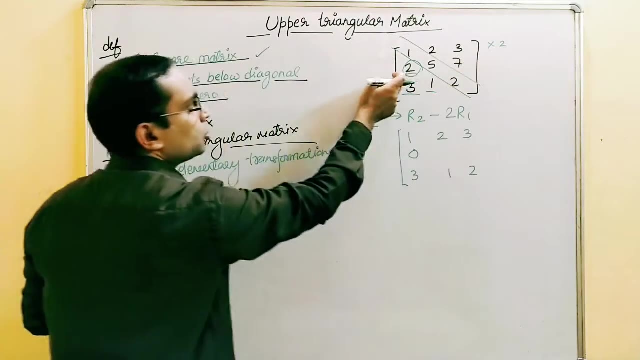 with row number two, so the resultant matrix will be: row number one will remain unchanged. row number three will remain unchanged. okay, so this is two. so two minus two, this will be a zero. we are multiplying two in this, so we are multiplying with two in this. so two into two, that is zero. 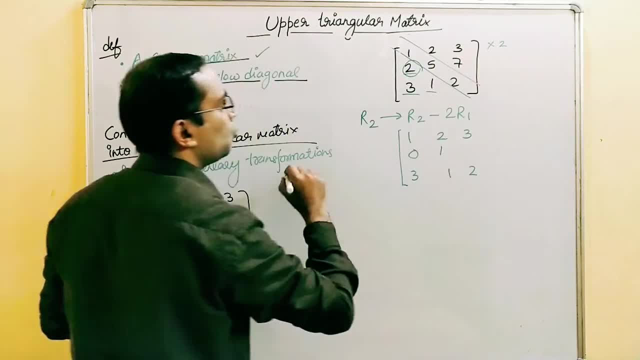 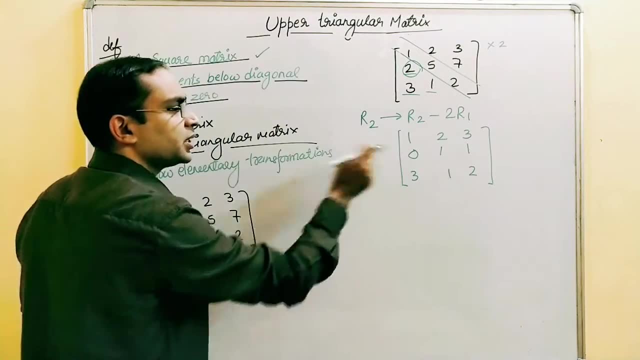 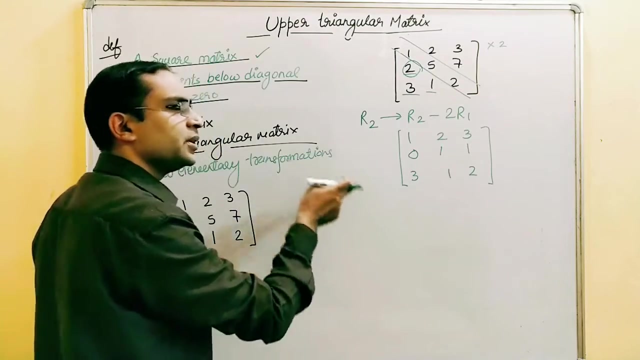 this is four: five minus four: this will be one. this is six: seven minus six: this will be one. so this is the first step, and we have converted this first element to zero. now we need to move down in the same column. first of all, we'll convert all the elements of that same column. 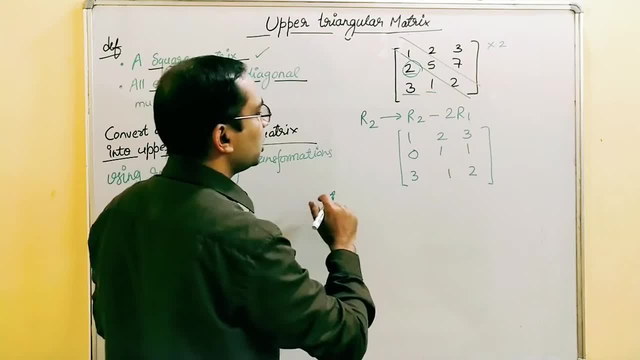 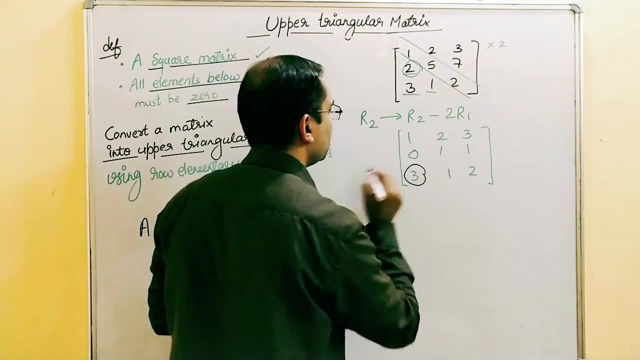 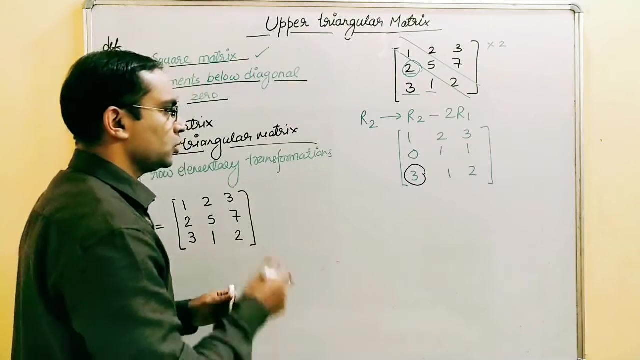 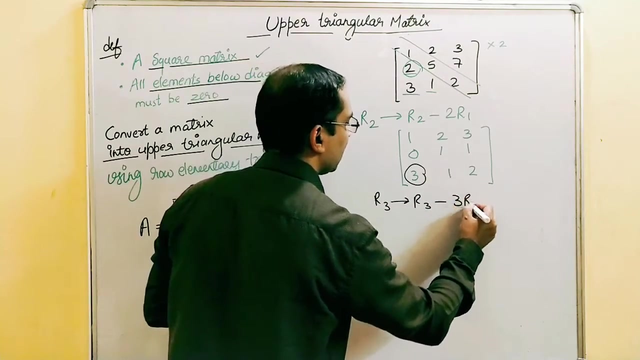 then only, we will shift to next column. so now we need to convert this next element in the same column. we'll convert this to zero, and again, this is in column number one, so we need to perform operation with row number one. so now, what will be the operation? so row three will be converted. so we'll subtract by three r one that. 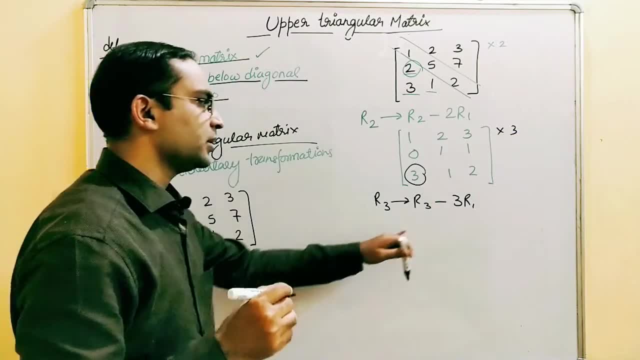 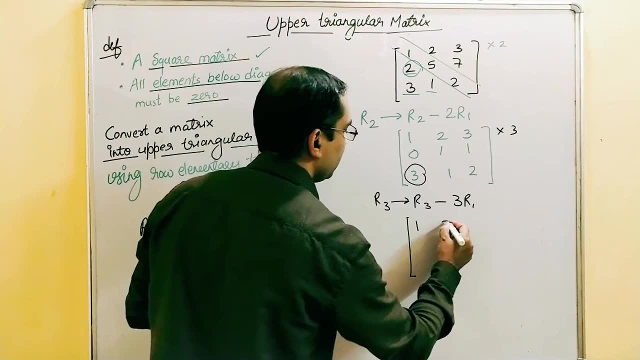 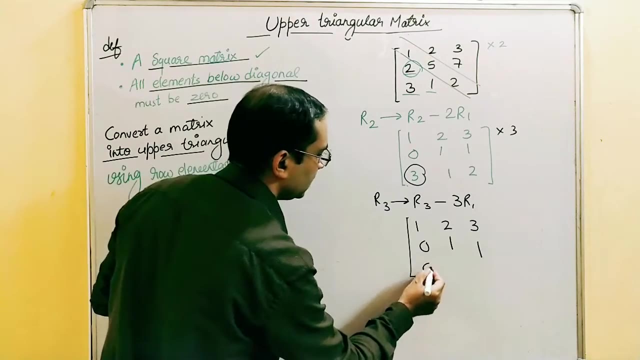 means we'll multiply by three in row one and then we'll subtract this from row number three. so now what will be the resultant? the next resultant will be: this will remain same: one, two, three. this will remain same zero. one and one. now, this is three minus three will be zero. one minus three to the six. so this is one minus six, that is minus of. 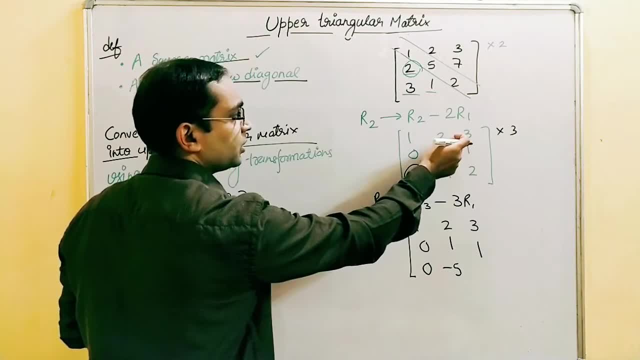 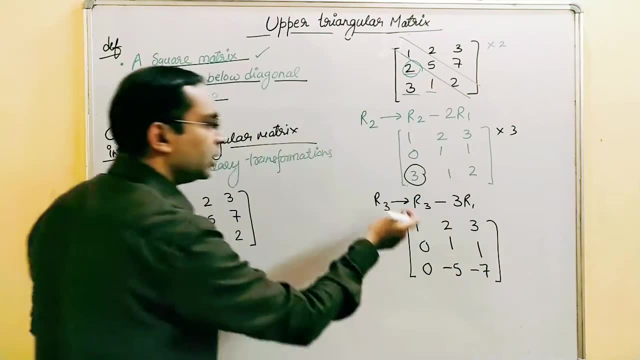 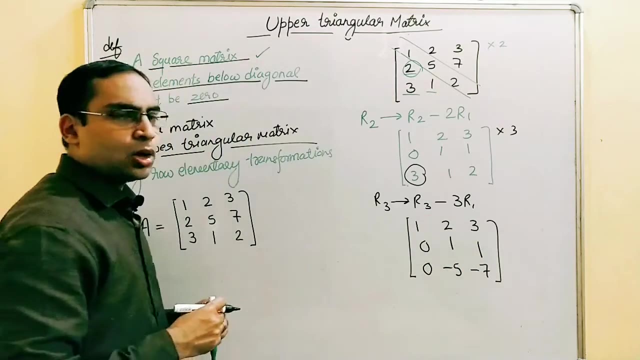 five, and now this is three to the six. three threes are nine, so this will be three. threes are nine. two minus nine, that is minus of seven. so we can see we have converted this element also to zero. now we have completed first column. now we can move to the next column and we need to convert only this. 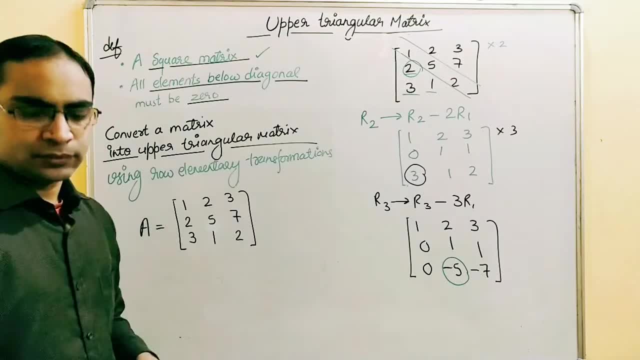 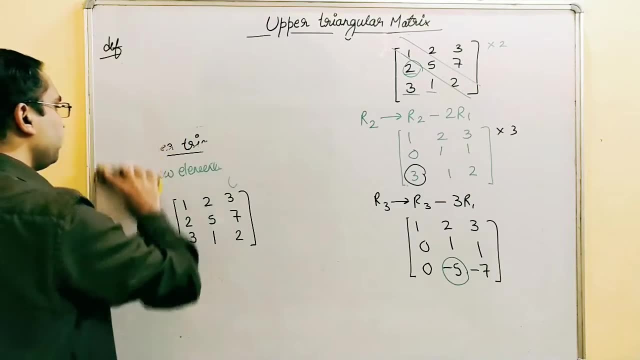 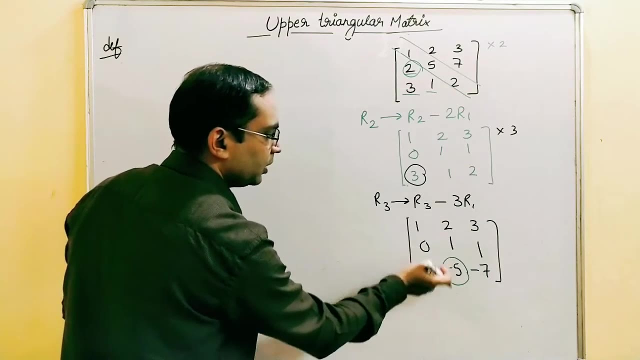 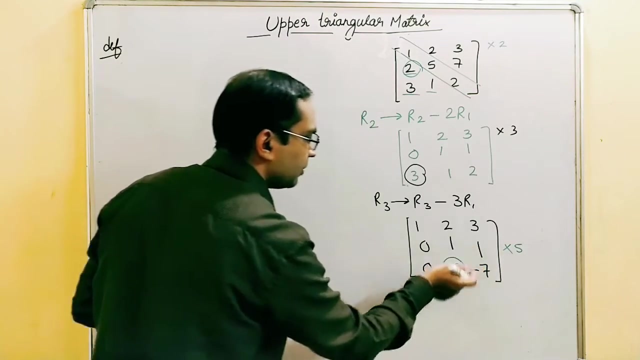 element to zero, that is minus five. so, just to convert this element to zero, what we need to do? uh, just remember, we need to perform operation with the row number two, because this element is column number two. so we'll perform with row number two. so what we can do is we'll simply multiply this by five and we can add both. 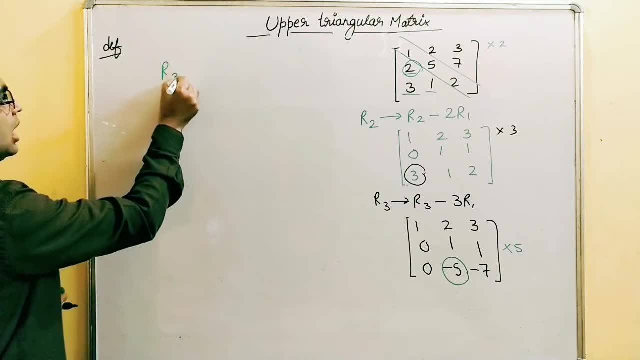 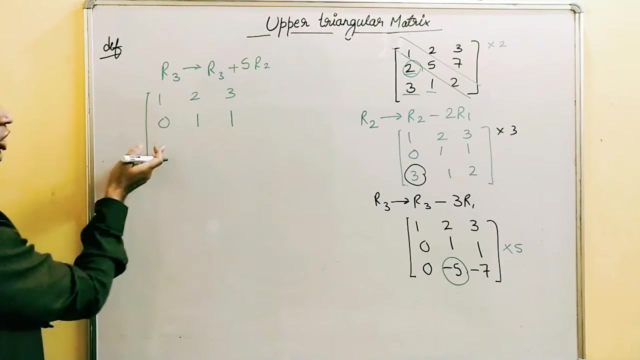 these rows, so the operation will be: r3 will be converted by r3 plus uh, five r2, so this will be the operation. the first row will remain same, one, two and three. second row will be same: zero. one and one third row will change. zero will not reflect, so this will zero. that is why 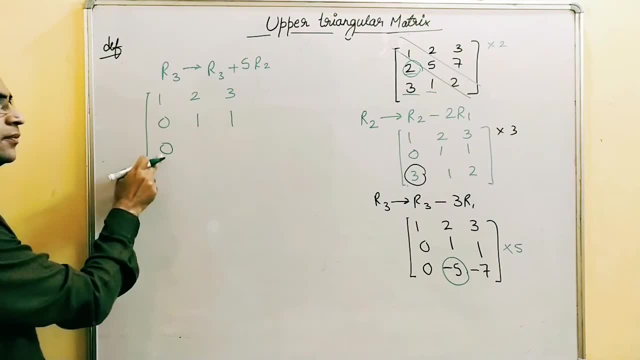 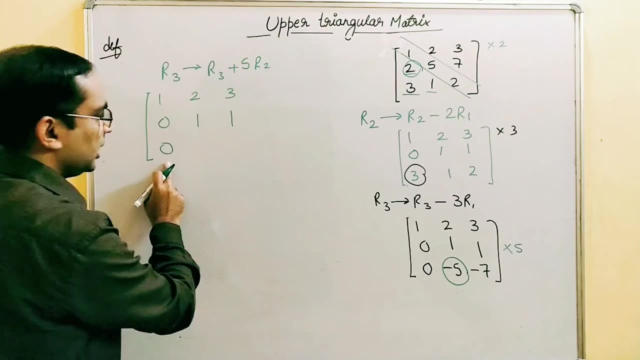 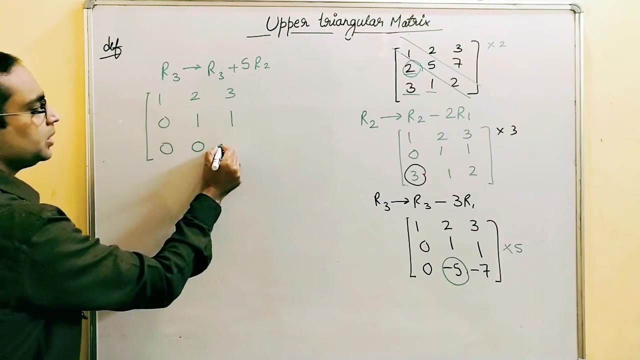 I have given you a particular order so that the element we have already converted to zero does not changes back to some other number, so it will remain zero. and then this is minus five plus five will be a zero. now, this is minus seven plus seven, will be sorry. minus seven plus five will give you a minus of two. 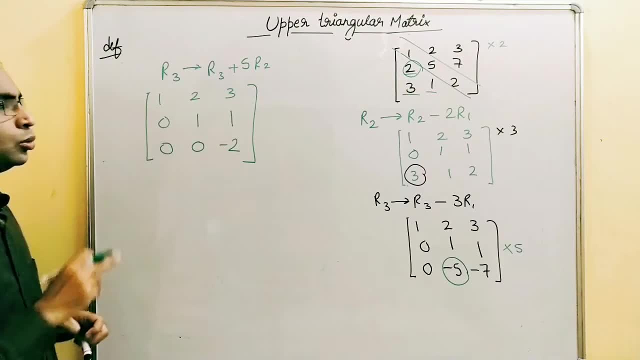 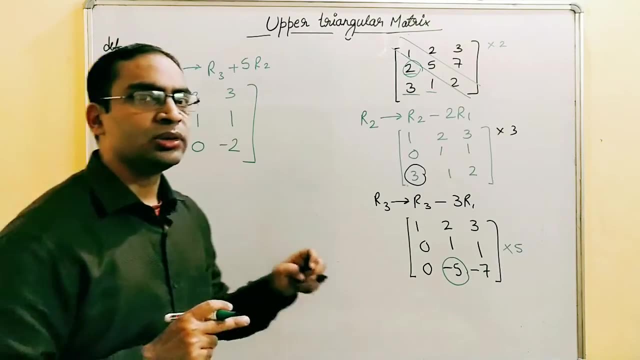 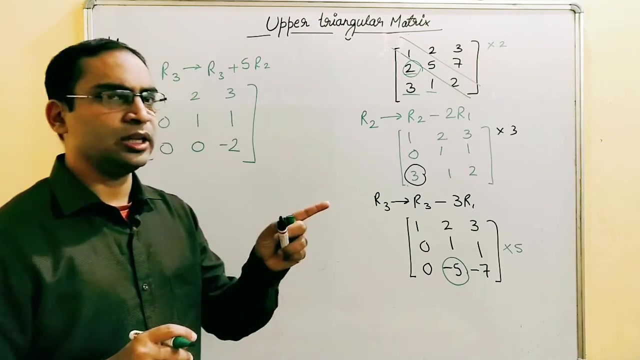 so now we can see that this is a matrix converted to upper triangular matrix. I hope you have understood the concept, uh making your mind that you need to follow these three steps so you can see. if you want to uh see that lower triangular matrix, I'll give you the link here and you can. 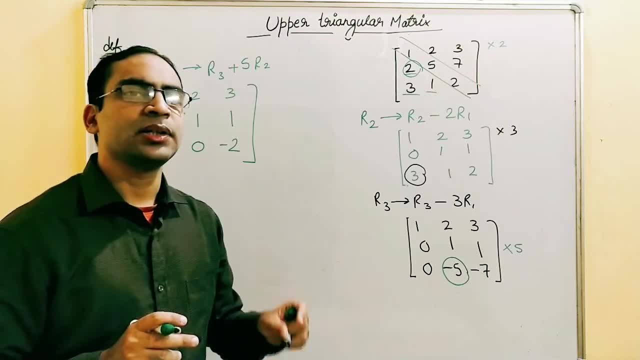 click on it and then you can see how we can convert a matrix into the lower triangular matrix. thank you so much.